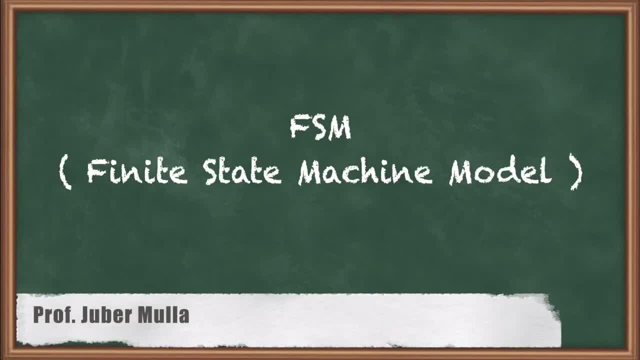 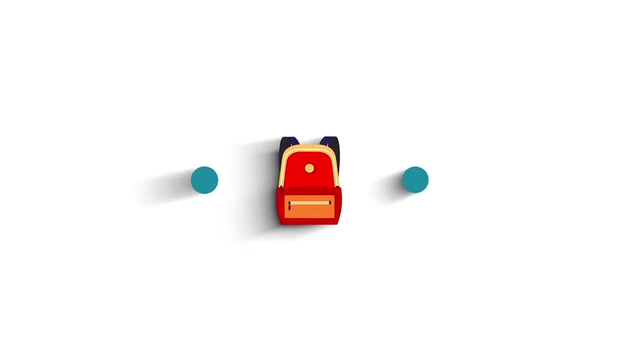 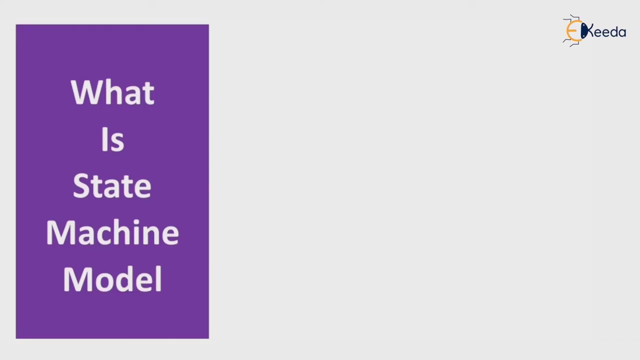 Hello friends, today we learn finite state machine model. The first point of discussion is: what is a state machine model? then a finite state machine model with one example. Let's start with what is state machine model? This is a reactive or event driven model or embedded system whose processing behavior 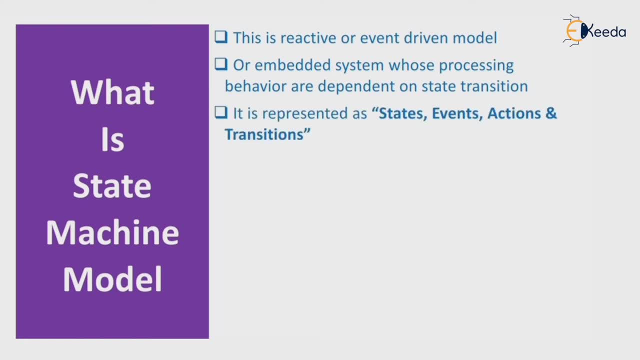 are dependent on state transition. It is represented as states, events, actions and transition. First of all, state State: it is representation of a current situation. event, it is representation of input to the state. action is a representation of activity to be performed by the state machine and the transition: it is the 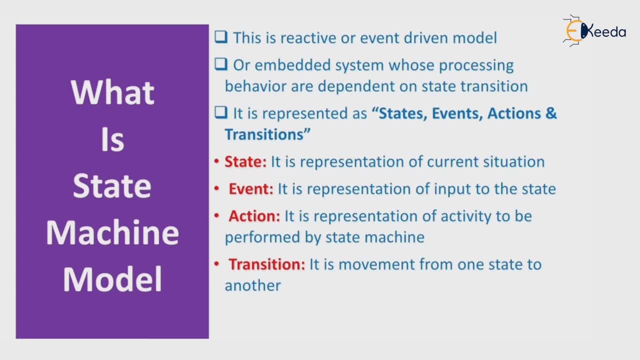 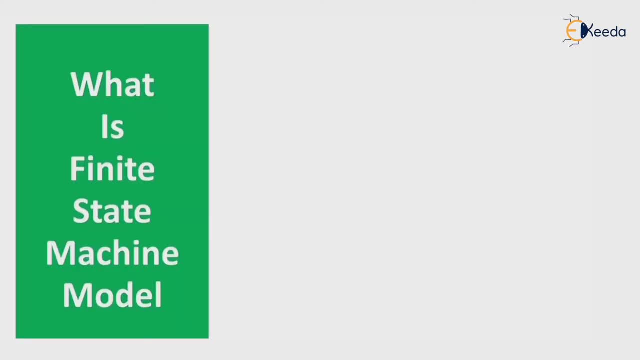 movement from one state to the another state. In that way, you can represent a state machine model. Now let's see what is finite state machine model: A model which is in which the number of states are finite. it is a model in which number 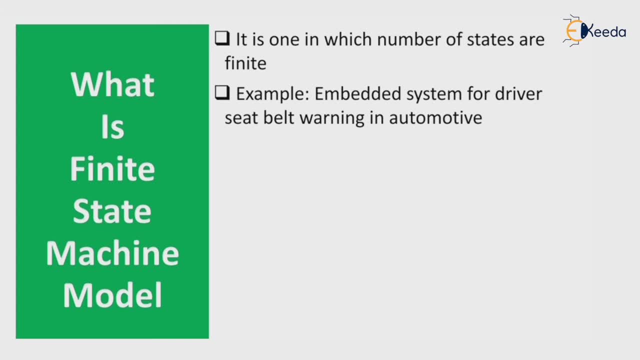 of states are finite, For example, embedded system for driver seatbelt warning in automobile or automatic car system. This is a finite state machine model in which include alarm on state, alarm off state & alarm reset on state. There are several examples of cheat modes. cheek mode can be height mode. There is one. orails state to indicator an alert and integrand on state. This is a finite state machine model which includes alarm of state etc. B3 keeps always function in the same location for machine mode. Let's see. the last one is Anterog. if an input of this stateier. 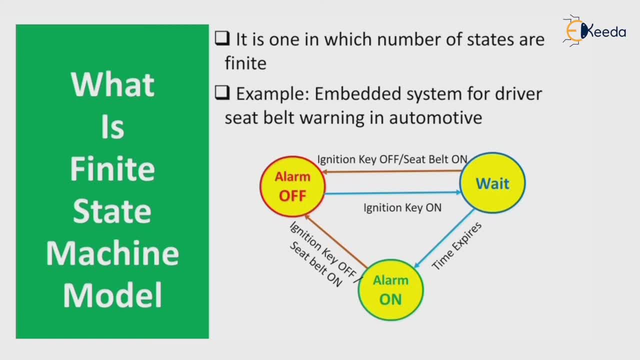 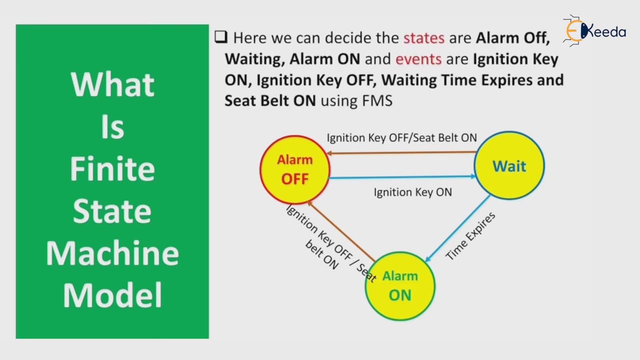 Alarm off, wait state and alarm on state, Depending on the seatbelt is on or off. the system is work Here we can decide the states are alarm off, waiting alarm on and events are. ignition key on, ignition key off, waiting time expire and seatbelt on using finite state machine.